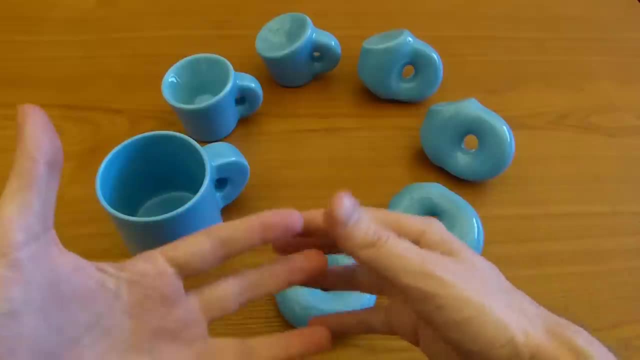 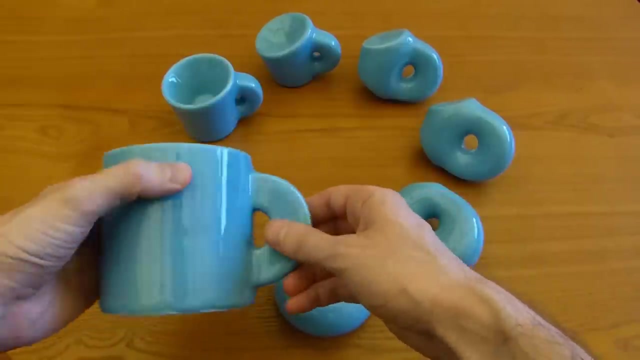 when you don't care about lengths and you don't care about angles. All you care about is the sort of global shape properties, And so everything's made out of very stretchy rubber, And in particular, that means that if you take a coffee mug, you can sort of unindent the place where the coffee goes. 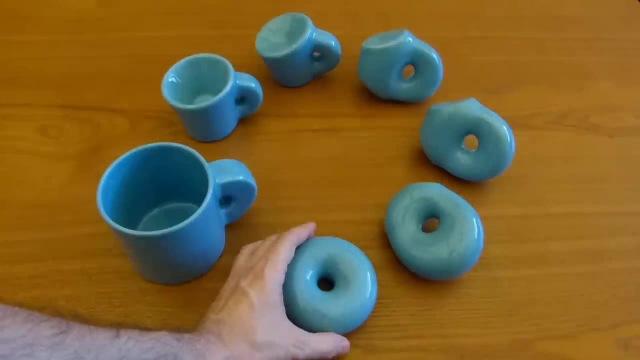 and you can kind of squish out the handle a little bit And eventually you can deform it into this perfectly symmetrical round donut shape. So, as the joke goes, the topologist doesn't know the difference between these, because in the study of topology you don't care about any of these. 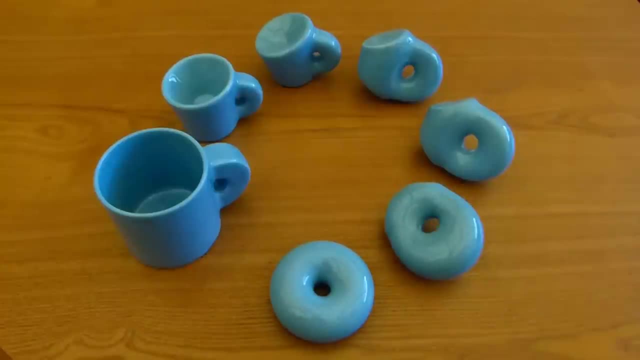 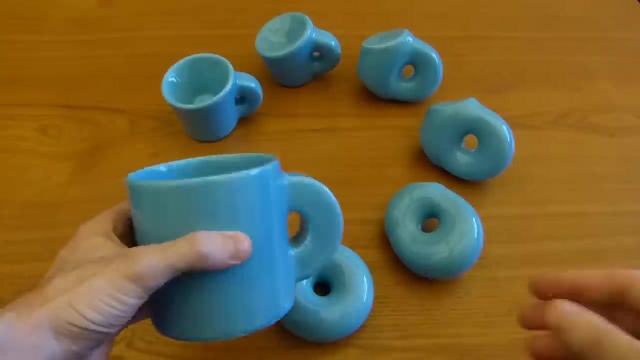 actual geometrical shapes of these different objects. So, as I say, this is joint work with Keenan Crane. He actually designed the shapes of these. I just did a little bit of editing to make them printable. Where do the shapes come from? Well, the thing you want to think about is soap films. So if you have, 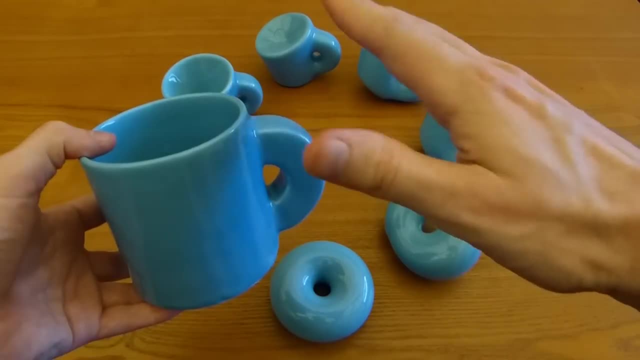 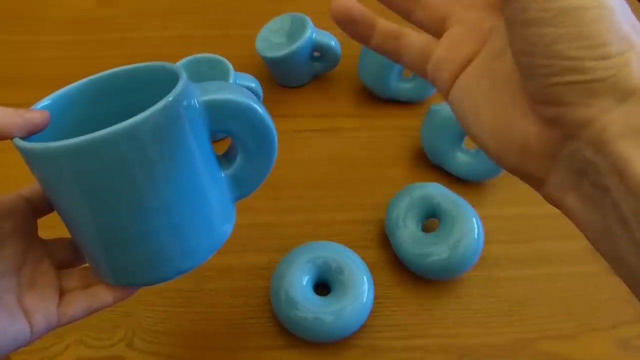 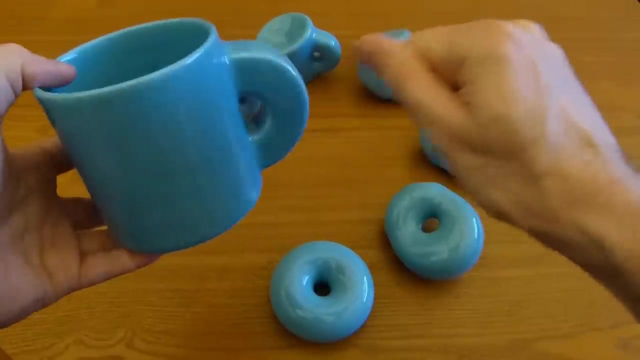 a soap film, perhaps not in the shape of a coffee mug, perhaps in the shape of a bubble, and you poke on it a little bit or you blow on it, then it gets out of shape and then it tries to snap back into this sort of minimal energy. The surface tension of the film tries to minimize its 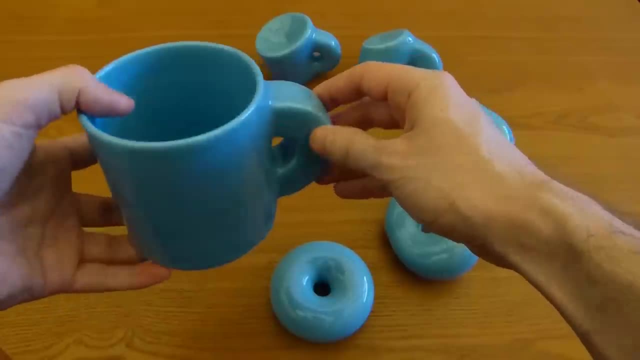 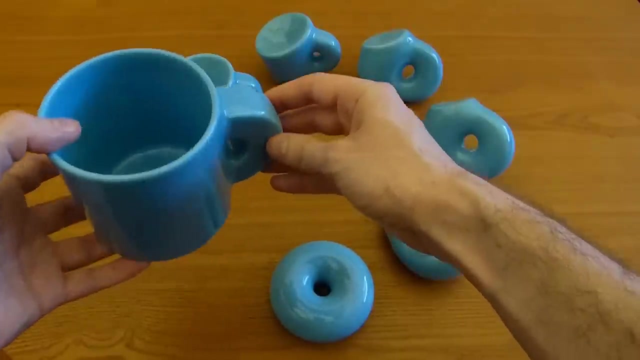 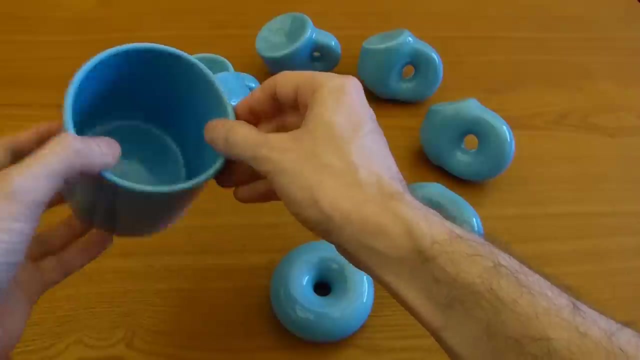 energy and change the shape so that it takes up the least area, And so there's a sort of energy that it's minimizing, And the same thing is going on here. So Keenan started with this shape of the coffee mug And then all these complicated features and sort of not terribly symmetrical shapes have 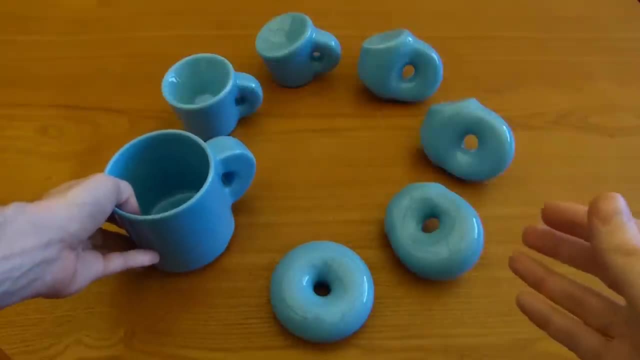